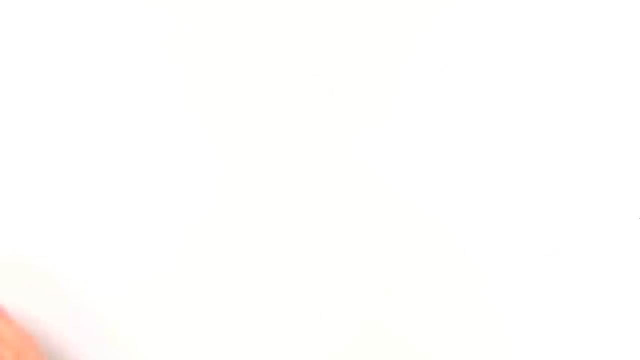 nations. Let's look at an example. Companies used to manufacture products in their home countries, just like the companies Profi TV and Supercolor who produce televisions in country A. Their products are in direct competition with each other, but both companies pay the same salaries and production costs. they have the same customers. 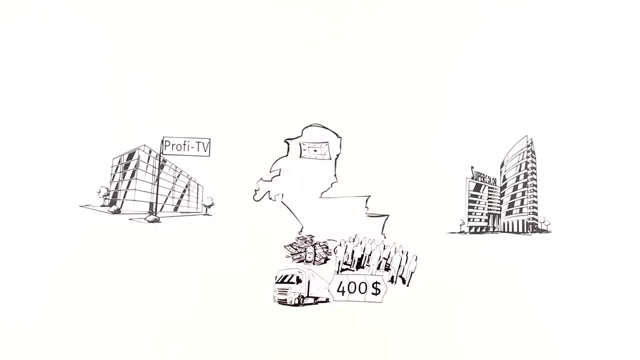 use similar suppliers and sell televisions at similar prices. In short, the same conditions apply to both companies. So far, so good. Due to technical, cultural and economic differences, economic developments that have come about through globalisation, other companies, which 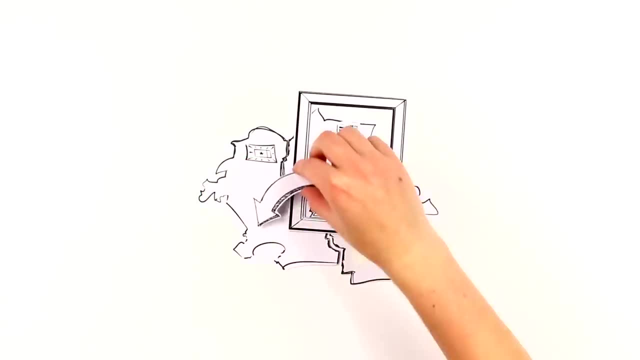 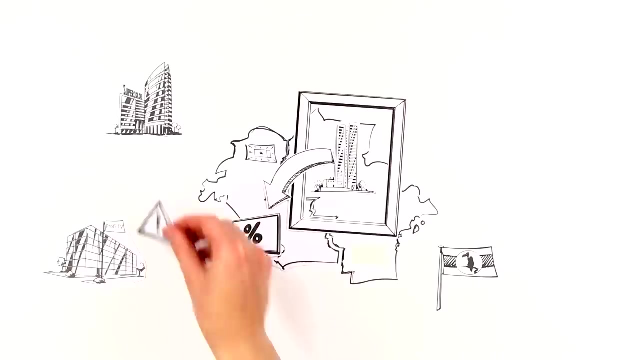 manufacture products under different conditions can now offer their products in country A too. That's why a company from country B can sell televisions here at a lower price because they were produced for less. The local firms Supercolor and Profi TV have to react to withstand. 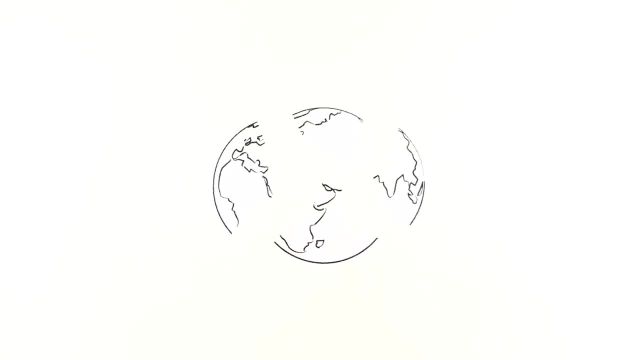 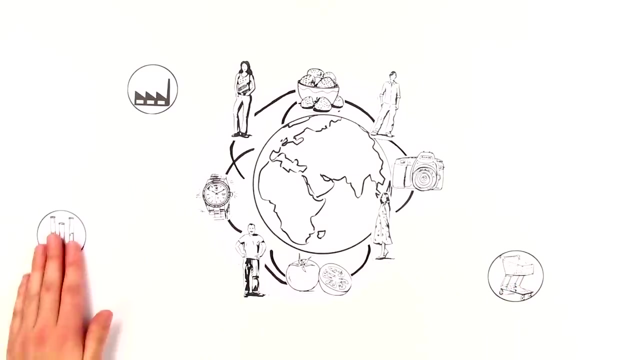 the competition, And so the world grows closer together and there is an active exchange of goods between countries. More affordable products are available for more people. However, not only does an exchange of products and economic goods take place, but also of services, knowledge, cultural. 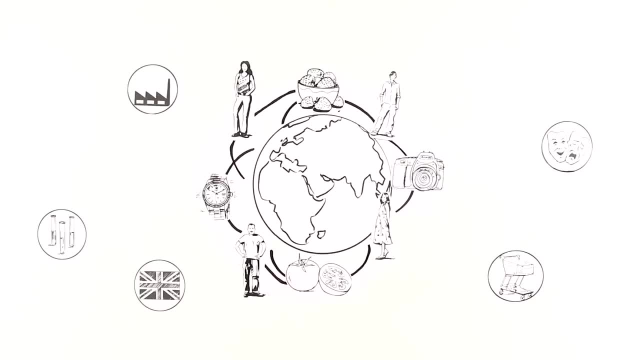 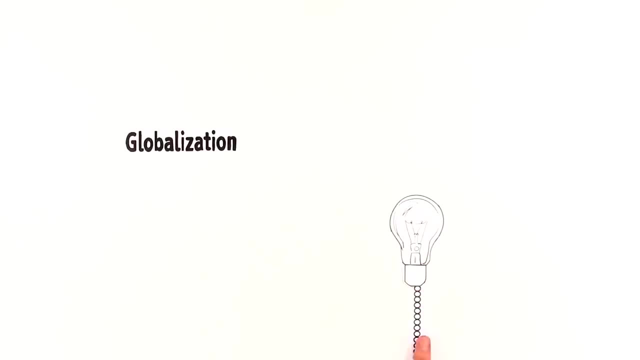 goods and even languages. All of these individual elements are closely linked and influence each other. But where there is light, there is also shadow. Because of globalisation and this intense exchange of goods, people and the environment often suffer If a company decides to move production to an economically disadvantaged country. people, in industrialised countries lose their jobs. At the same time, job opportunities open up to many locals in the economically disadvantaged country. Many people in these countries work for very little money in comparison to those in industrialised countries. Therefore, they often remain poor and, more often than not, do not have sufficient insurance, social insurance. 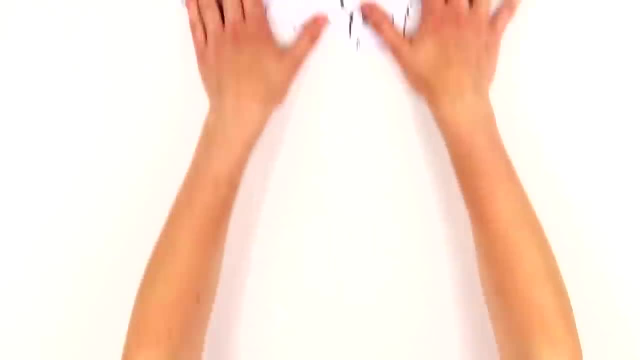 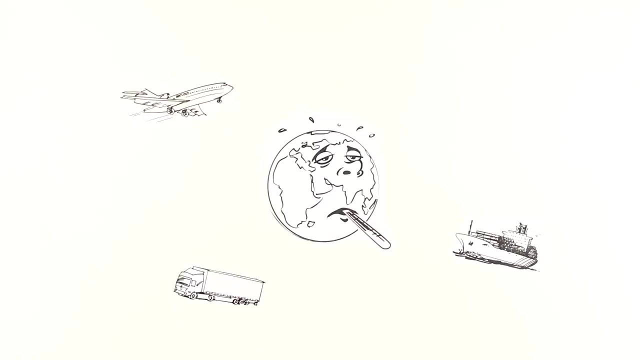 or health insurance cover. A further disadvantage of globalisation is ecological problems such as climate change. The use of aeroplanes, ships and lorries to transport goods over international borders is constantly on the increase. This causes more carbon dioxide to be released into the.